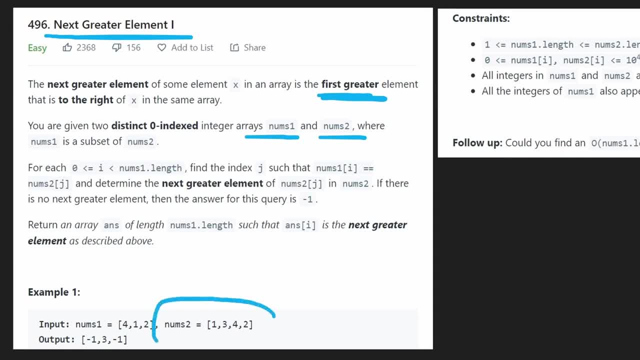 little bit tricky to understand. So if we were just given this array of nums one and nums two and we had to find the next greater element of every single value in this array, that's simple to understand. But what the problem is asking for is actually a little bit more complicated than. 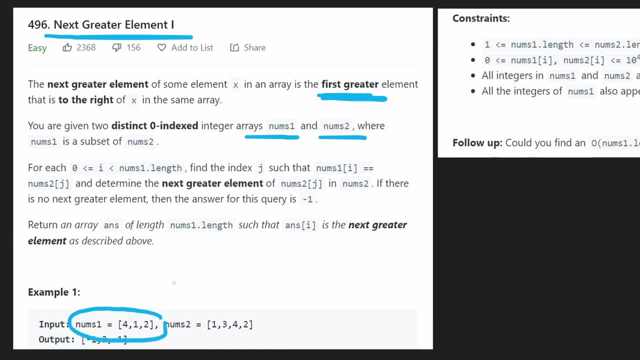 that. So basically, since nums one is a subset of nums two, we actually only want to find the next greater element of the values in this array that are also included in the first array. So we don't want to find the next greater element of every one of these, So we're going to have to find the. 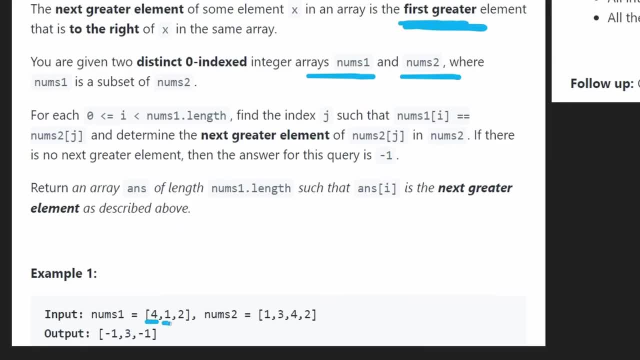 only want to find the ones that are four, one and two. So four, one and two, you can see that they don't even show up in the same order, So that's going to be a little bit annoying, And so the output that we return is, of course, going to be the same size as nums one and the order of the. 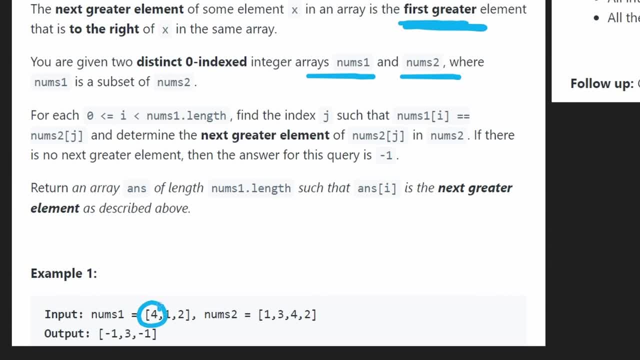 values is going to be the same. So if we want to know the next greater element of four while we look at our second array, four is over here. What's the next greater element of it? Two is not greater than four and there's no other elements here, So four doesn't have a next greater element, So the. 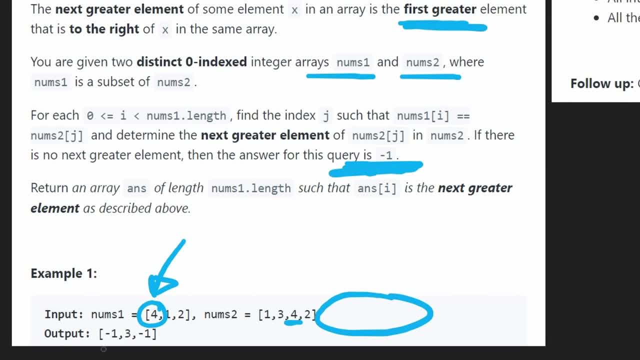 default value that we do in this case is going to be negative one, So we just put a negative one in the output. The next value is one. What's the next greater element of one? Well, looking at the next value, three is greater than one, So that is the next greater element of one. Four is also greater. 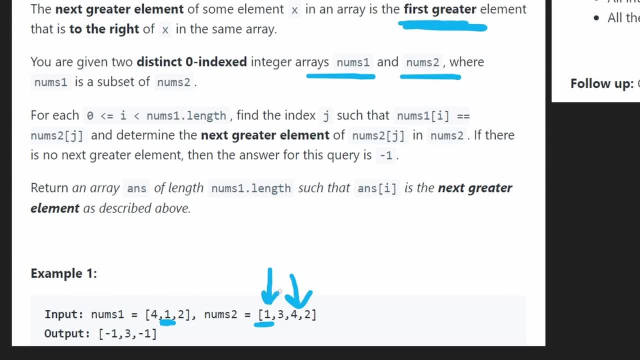 than one. but three is closer to one on the right side, So we use three in the output For two. two doesn't have any output, So we use three in the output. So we use three in the output. So we use three elements to the right of it so it doesn't have a next greater element. We can just put. 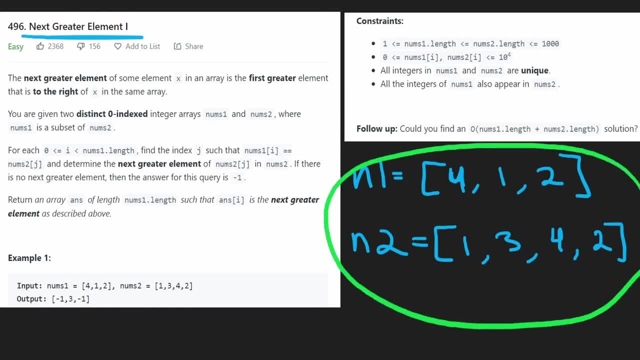 negative one there. So the brute force of this problem is not super crazy, but it's a little challenging for an easy problem. So one way to approach this problem is to kind of just find the next greater element for every single one of these, because we know if we do that we'll pretty. 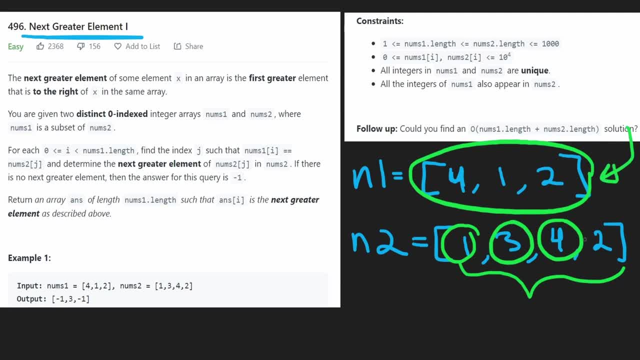 much have what we're looking for, and then we can create the output. But at the same time, we could also skip the values. we don't need to. In this case, three is not in the first array, so we don't need to find the next greater element of three. So what I'm actually going to do is convert the. 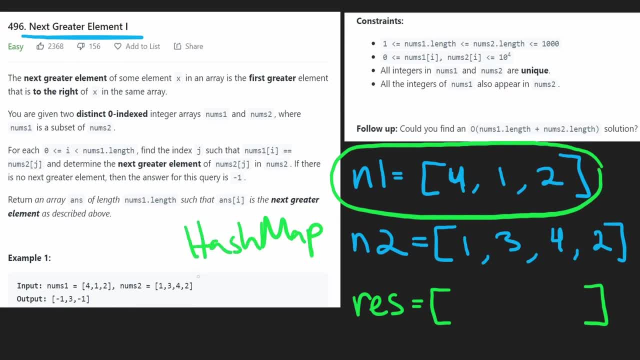 first array into a hash map where we're going to be mapping every single value in that array to the index that it shows up in in the same array. The reason we're going to be doing that is because, let's say, we are iterating through each value in n2.. So we have one. So first we would 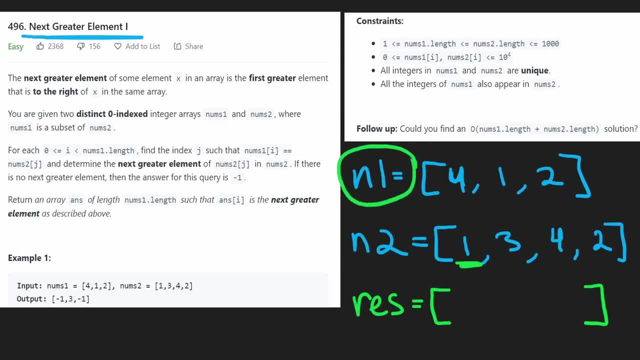 want to know: does one even show up in the first array? Yes, it does, So we're going to do that. Okay, so we need to find the next greater element of one. Let's say we find it over here. three: Okay, we found the next greater element of one, So now we want to add that three to the output. 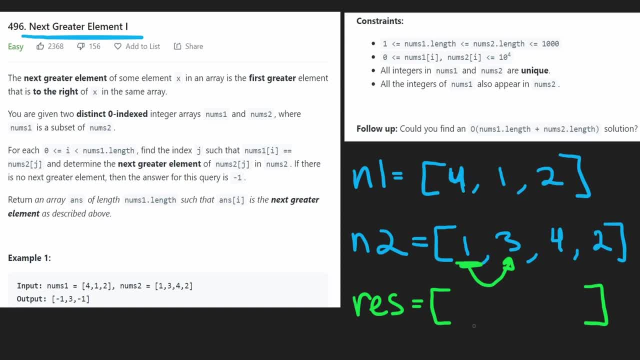 in our result. Well, where are we going to add it in the result? Are we going to add it here or here or here? Well, it depends. where did one show up in the input array? It showed up over here at index one, So that's going to be the same index we added in the output. So that's why we 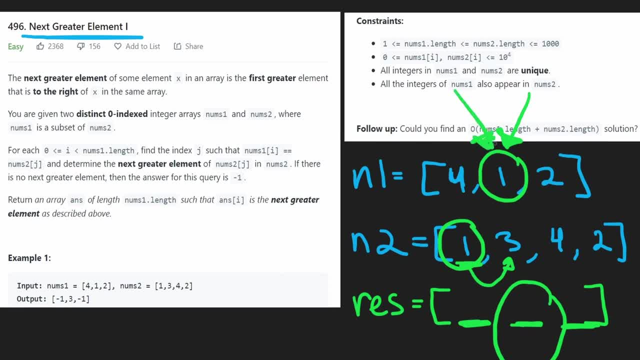 need the hash map so that we know that we're going to be adding it to the output. So that's why we need the hash map, so that we know the index of every single value. And the hash map will also be very efficient for us to just look at this value and say: does it even show up in the first? 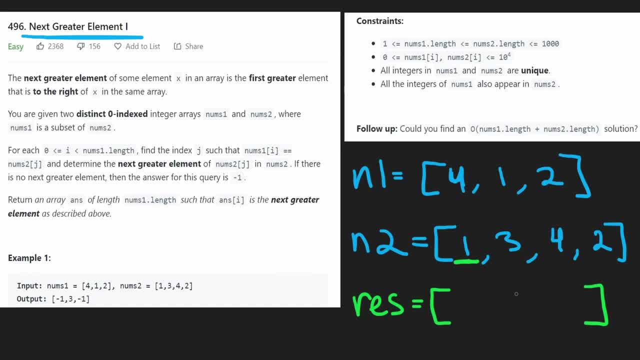 array Yes or no. We can do that in o of one time. Okay, so we we found that that's, you know, the next greater element, And then we're just going to basically repeat that for the rest of the array. So three: does it show up in n1?? It does not, So we can skip it. Four: does it show up in n1?? Yes, it. 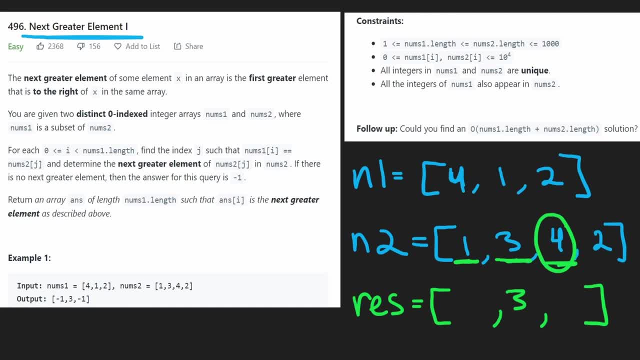 does So we can't skip it. And how are we going to find the next greater element? Well, pretty much, we're going to iterate through the index of every single value. So we're going to do that in the entire array until we find a value that's greater than four. The first value that we find, that's: 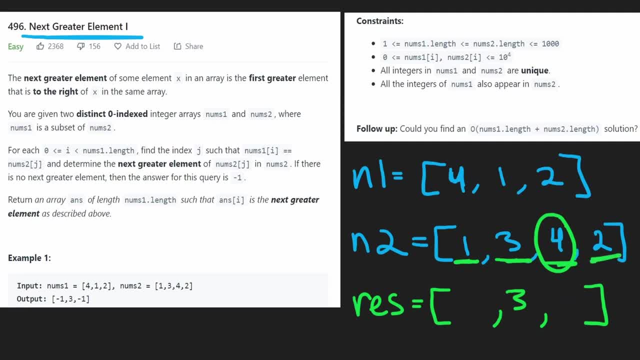 greater than four and then add it to the output. But in this case we would iterate through it and see that it doesn't exist. So in that case we could just add a negative one in the same corresponding position. But we could also just initialize our result array with all negative ones. 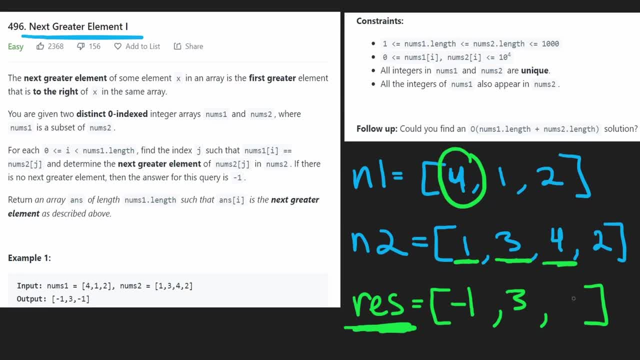 so that we don't even, you know, have to do that, Which is probably how I'm going to handle it in the code. And then, lastly, for two. there's no other elements that come after two, So we'll just add a negative one here. So not super crazy, But the overall time complexity, if you kind of caught it. 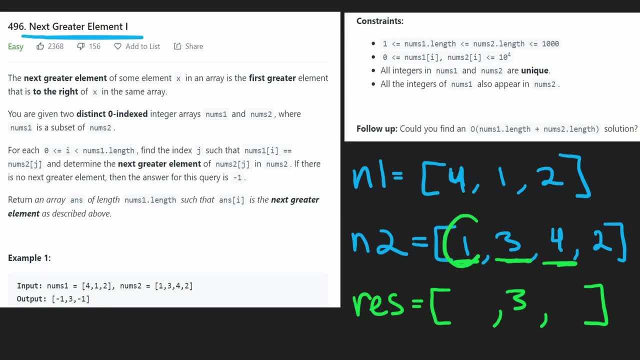 is going to be n squared Because for every single value in n2 we're potentially going to have to iterate through the entire input array to find the next greater element, And we're going to have to do that for every single value in the array in the worst case. So the time complexity is going to. 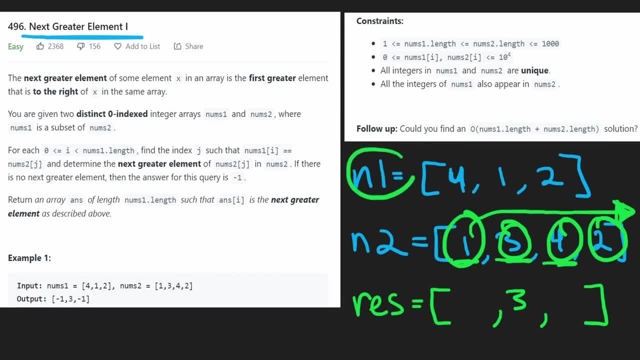 be something like n squared, But technically, let's say, the size of this array is m and the size of this array is n. Technically, I think the time complexity is actually going to be n times m, Because we're not finding the next greater element for every value in this array. We're only doing 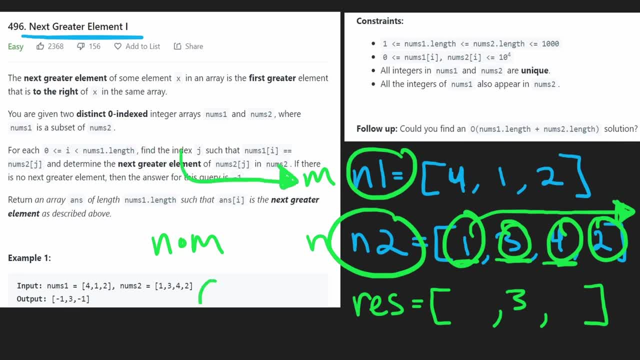 that for every value in the first array The memory complexity is going to be big O of m, Because we're going to have a hash map for the first array And we're also kind of building the output as well. So now let me just show you the code really quickly And then we're going to get. 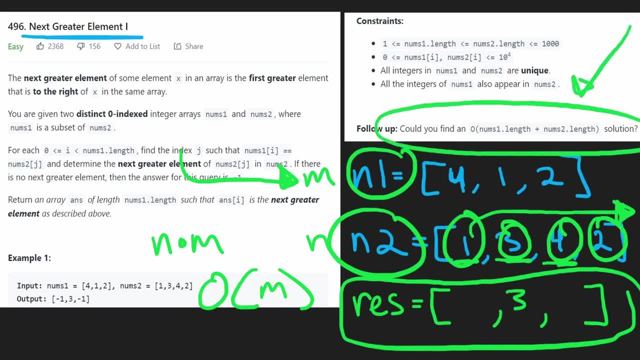 to the more complex solution, But also the more efficient solution. Okay, so let me just show you the code really quickly, And then we're going to get to the more. So let me just walk you through the code really quickly. So, like I said, this is going to be our. 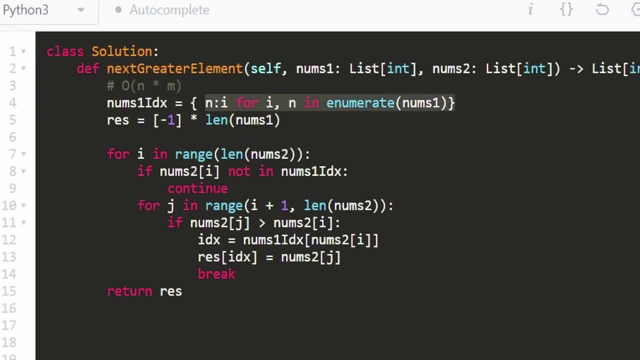 hash map. The way I'm initializing it is kind of you know some Python fancy stuff, But you don't have to do it this way. You can do it a traditional way if you want. But pretty much this is just taking every single value in nums one, mapping it to the index that it shows up in, Then we're. 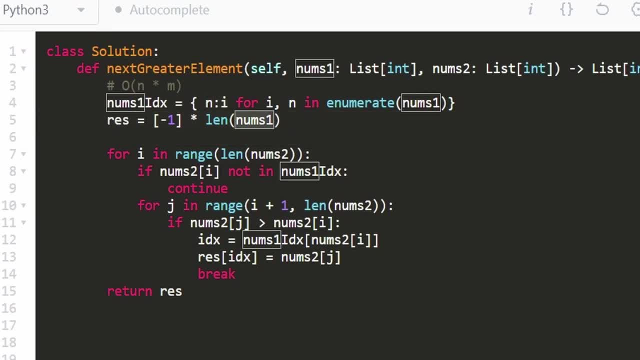 having our result, which is an array of the same length of nums one. Initially it's just going to be all negative ones, Because we know that's kind of the default value, And then we're basically doing our nested for loops that I talked about. We're going through every value in nums one. 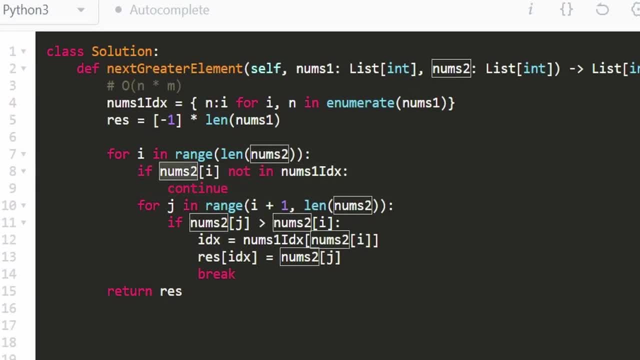 And then we're checking if it's going to show up in nums two, The bigger array. But we're checking: does that value even show up in nums one? If it does not, then we're just going to skip this value and then go to the next iteration of the loop. But if it does show up, then we're going to do our. 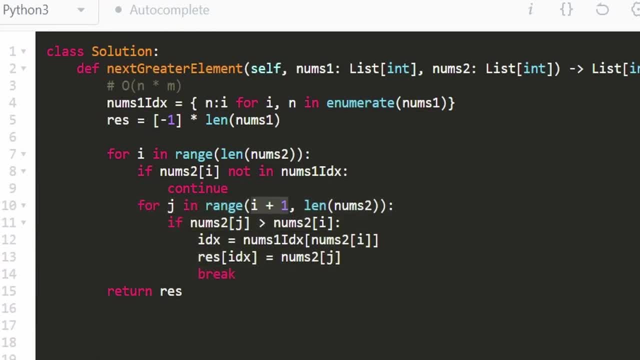 nested loop. Then we're going to go through every single value, starting at i plus one, Because we only want to look at the values that come after the original value, And then we're checking which is the first value that's greater than the value that we started at. If we find the next greater, 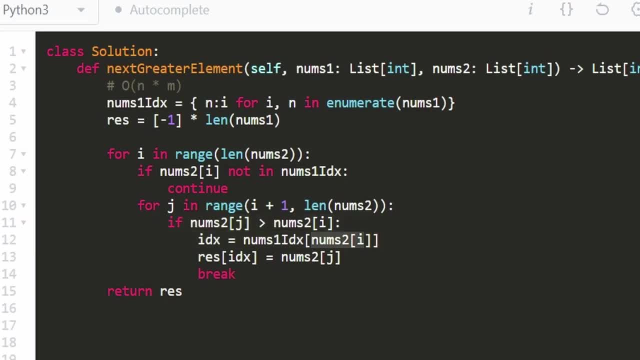 value we're going to get, first of all get the index of the original value And then we're going to set the result equal to the next greater value And then break out of this loop because we're already done. But if this never executes and we never find the next greater element, then the 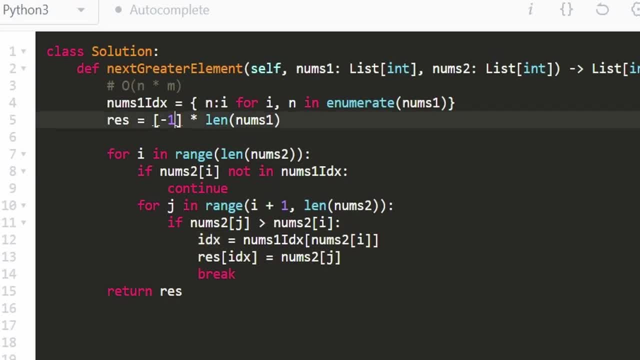 result will stay the same at that index. It'll stay as a negative one, the default value. So that works out for us. And then, once this nested for loop is done, we'll just return the result. So that's the basic brute force solution. Now let's look at the more complex 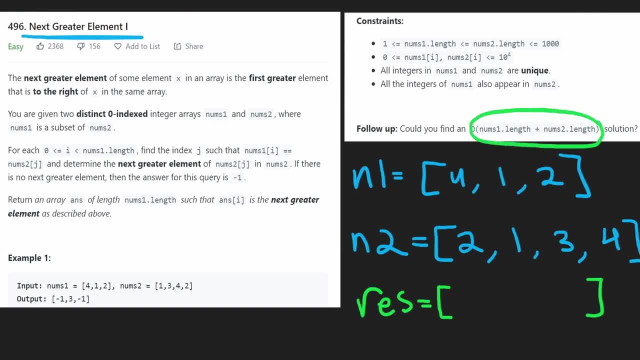 More efficient one. So now let's look at the n plus m time solution, And I'm just going to tell you straight off the bat that this is going to take a stack to solve. But it's not super intuitive to know that it's going to need a stack, Especially if you never solved this type. 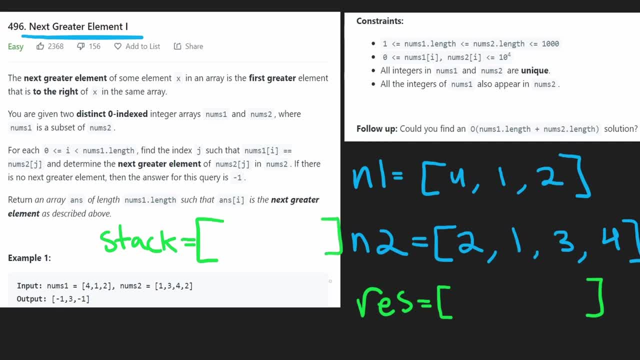 of problem before If you've never heard of the monotonic stack technique, But I'll try to explain the intuition of why I changed the example a little bit though, because the original example doesn't really lead to the intuition of a stack. So that's why I changed the. 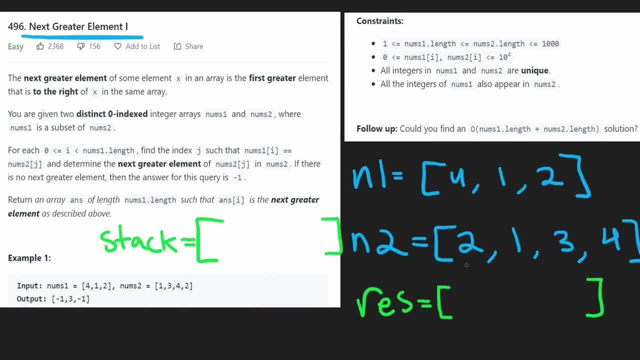 the order of the stack. So that's why I changed the order of the stack, So that's why I changed the order of the values, at least to this, because this will be a bit more interesting. So let's say we started at two. We know two shows up in the first array, so we want to find the next, greater. 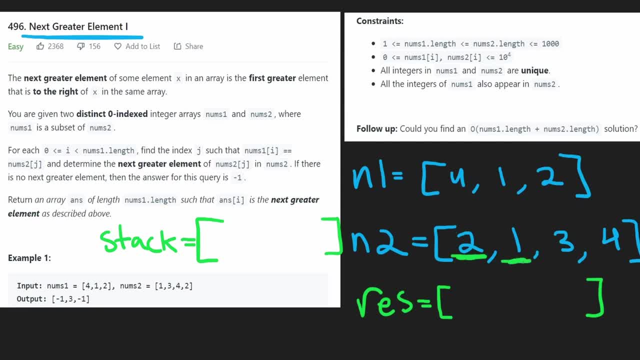 element of two. We look at the next value one: It's not greater than two, So it's not the next greater element. Then we look at the next value, three: It is greater than two. So we found the next greater element of two and we can add it to the output, But hold on a second If 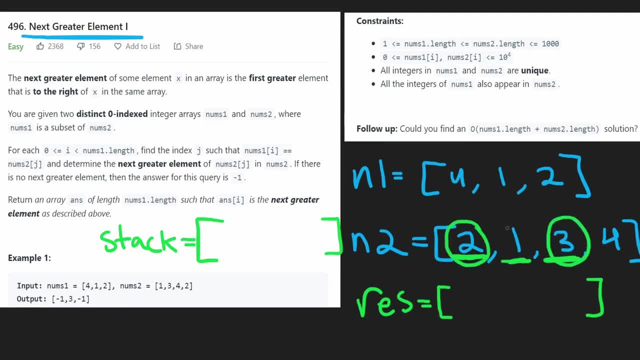 three is the next greater element of two, shouldn't it also be the next greater element of one? Well, that's only the case if one even shows up in the first array, which it does. But then that is the case, And that would be the case for any number of values You know, suppose before the three and 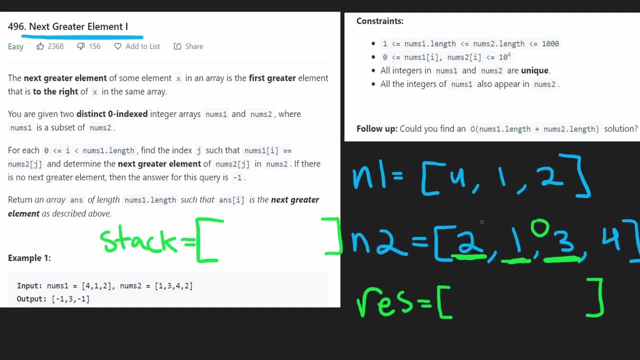 after the one, we had a zero over here. Then we'd say, well, one is not greater than two, and zero is also not greater than two. But when we finally reach the three, three is greater than all of them by definition, because all the values that came after two. 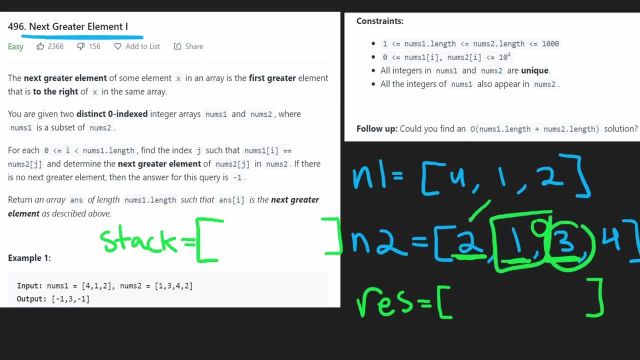 before three, they were definitely not greater than two. That means they must be less than two because all the values in the input array are unique. So that means when we find the answer for two, we're also finding the answer for all the values in between. That's where the stack. 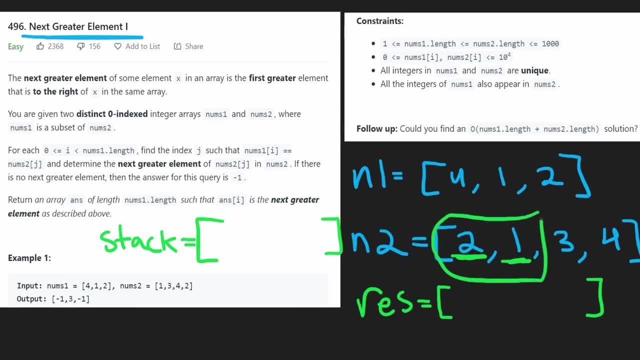 is going to come in, because we want to remember all of these values. In this case, of course, there's only two of them, but, like I said, there could be a lot more. So how the solution is going to go is: we're going to start at two. It's in num. 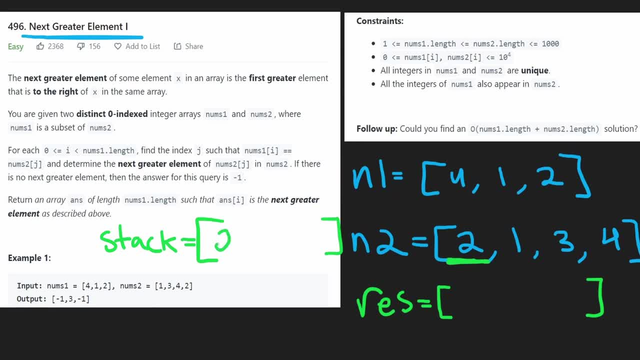 one. so what we're going to do is add it to the stack. You're going to notice that this is going to be a one pass solution. We're not going to have nested for loops. Next, we're going to look at the value one. First of all. is it greater than any of the previous values that we need to find the next. 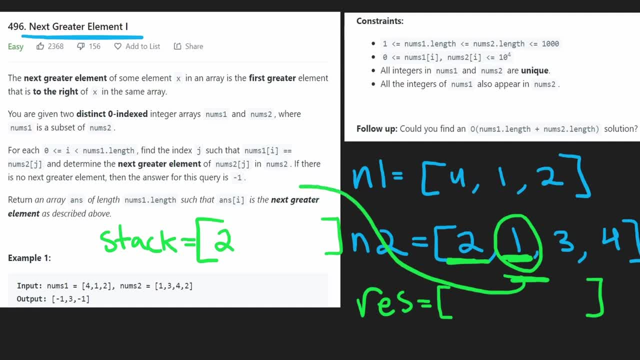 greater element for. Well, we're going to check that by taking the value one. So we're going to look at our stack. What's the top value on our stack? It's two, So one is not greater than that. So we didn't find the next greater element of two, But one does show up in num one, so we are going to add it to the stack because this is another value. we need to find the next greater element for. 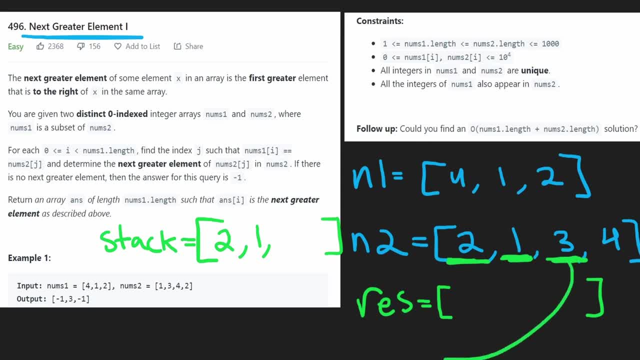 Okay, and then we look at three and we're going to compare it to the top value of our stack. Notice how the stack is always going to be in double. So we're going to look at our stack decreasing order. It has to be because, by definition, if we find a value like we just 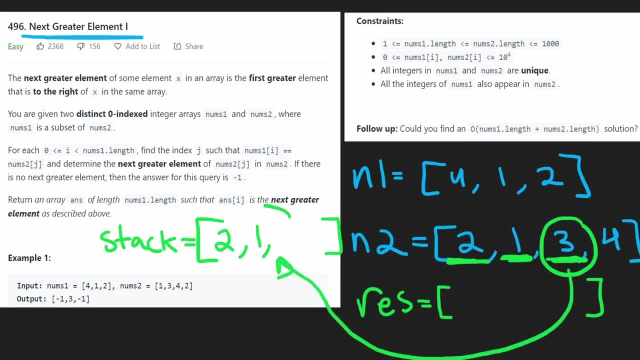 did. now we found a three and that's greater than the values here. So now what we're going to do is pop all of these values. What we're going to do is see three is greater than one. We found the next greater element of one, So what we're going to do is find the index of one. We're going to 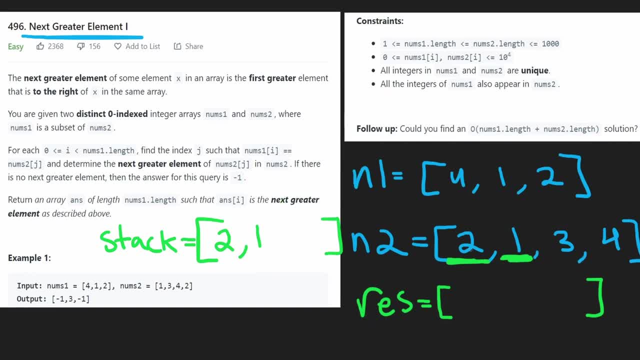 use the hash map that we talked about in the previous solution to do that. So we're going to say the next greater element of one is going to be three, And we're also going to pop this from the stack, And we're not going to stop there. We're not just going to check one value from the stack. 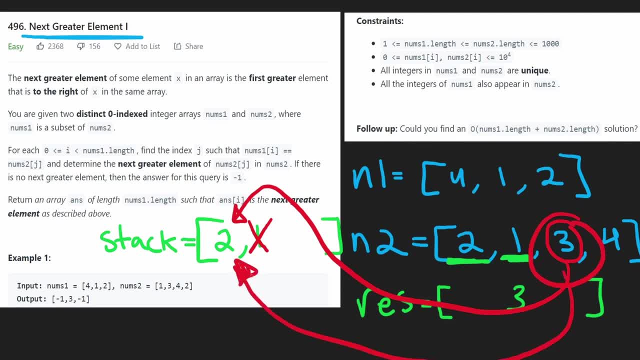 This three could be greater than multiple values on the stack. So what we're going to do again is compare it to two. Is three greater than two? Yes, it is, So we're going to pop the two. We know that two shows up at this index, So we're going to add a three at that index. We found the next greater. 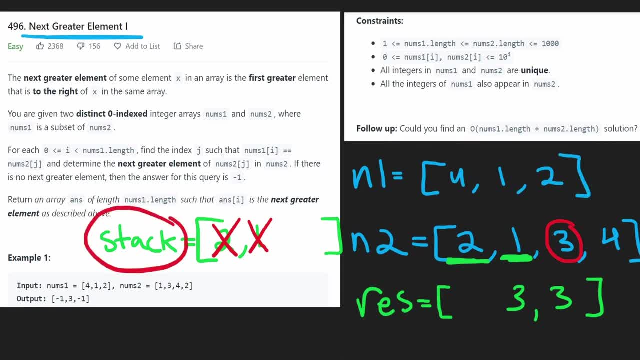 element of two, And now the stack is empty. So we can't keep, you know, popping values anymore. So we're done with that phase of the algorithm. Now is it time for us to add three to the stack? No, because three does not. 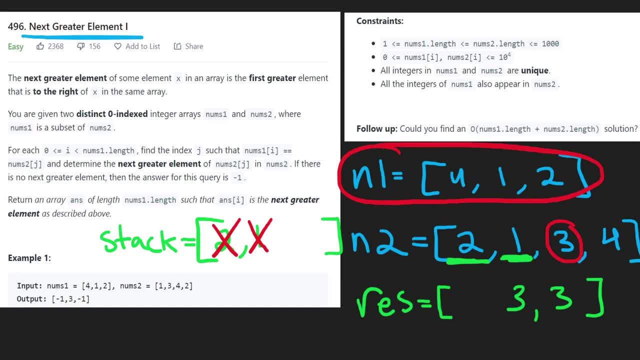 show up in the first array, So we don't need to find the next greater element of three. So we're not going to add it to the stack. So now we're done looking at three. We're going to go to the next value. four: We're going to add four to the stack. Then we're going to go to the next value. 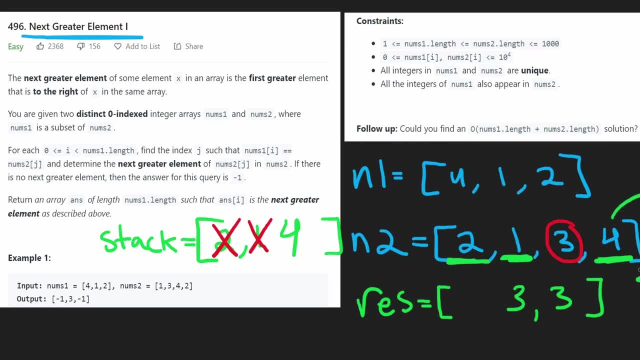 after four. Well, there aren't any values after four, So we're going to add three to the stack. So the next element for four is just going to be negative one, So we're just going to add a negative one at that spot. So notice how we did that, And we did it with one pass through the. 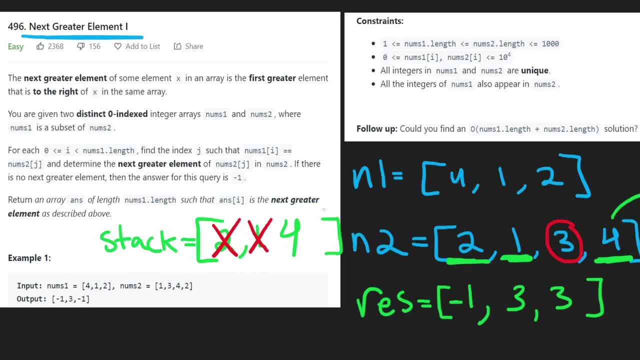 input array. Now we are adding elements to the stack, but we're also going to only be popping each element from the stack once. So the overall time complexity- yes, in this case- is going to be m plus n. The space complexity is also going to be a big O of m one because of our hash map. 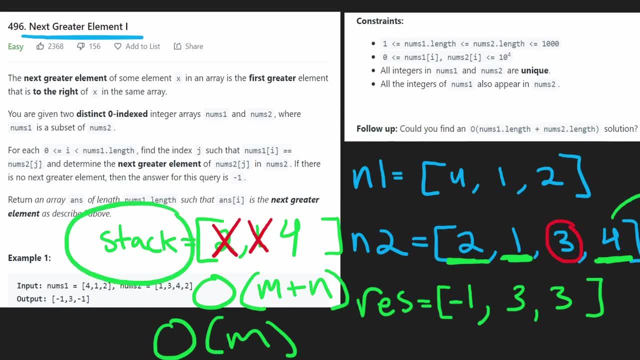 the size of the first array. Also, the stack is only going to be the size of the first array because we're only adding elements from the first array to the stack. So that's pretty much the whole solution. I really hope it makes sense. Now let's code it up. Okay, so now let's code up the. 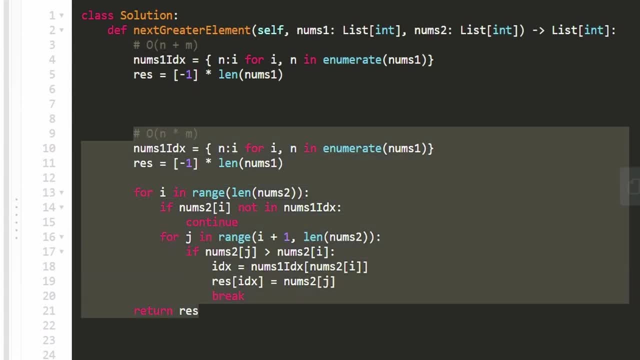 more efficient solution. You can see, I have the original solution down here And we're going to be starting this problem the same way that we did. We're going to have that exact same hash map and initialize our result the exact same way, But in this case we're also going to have a stack. 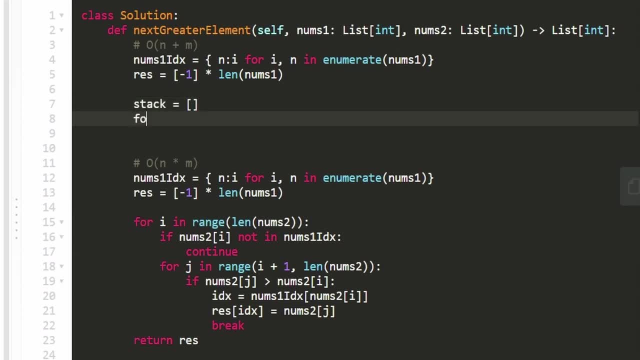 which, initially, is going to be empty, just like the drawing explanation, And then we're going to start iterating through every element in the second array, just like we did in the first solution. But where things are going to get a little bit different is we're going to look at? 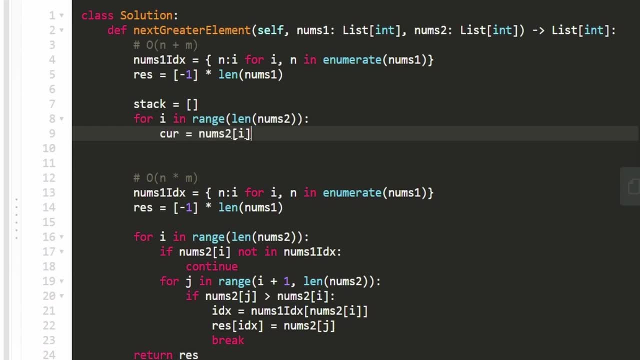 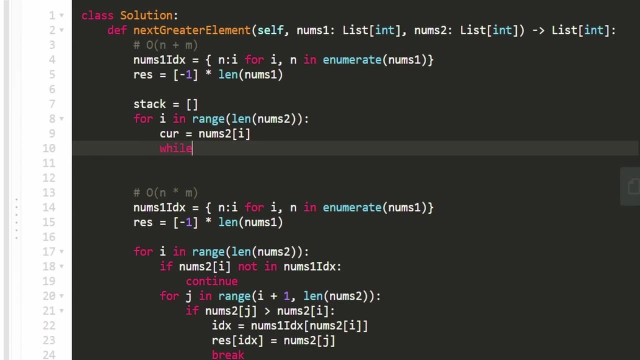 the current value, which is just nums two at index i, And we want to know if this is the next greater element for any previous values that could be on our stack. Now, initially our stack is empty, but later in the algorithm it could be non empty. 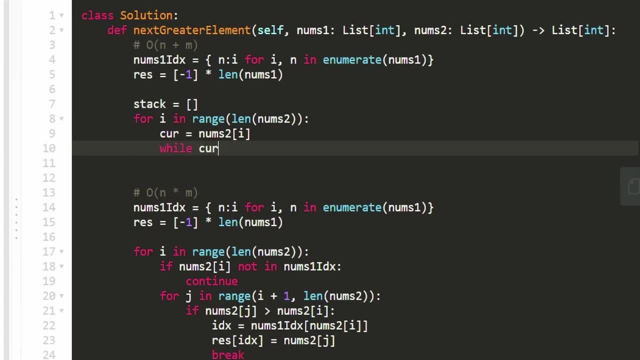 So in that case, if it was non empty, we would want to know: well, is the stack non empty and is current greater than the top of our stack? the top of the stack you can get with a negative one in Python, or you could take the length minus one. If this is the case, of course, 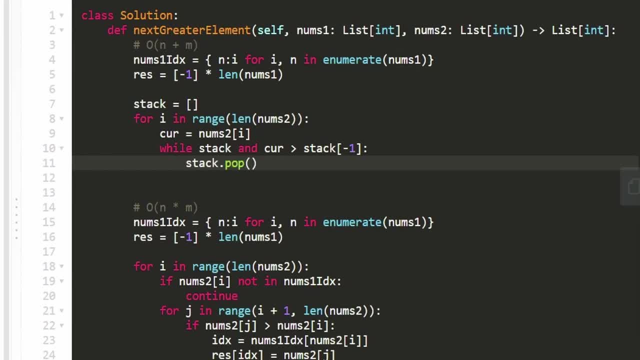 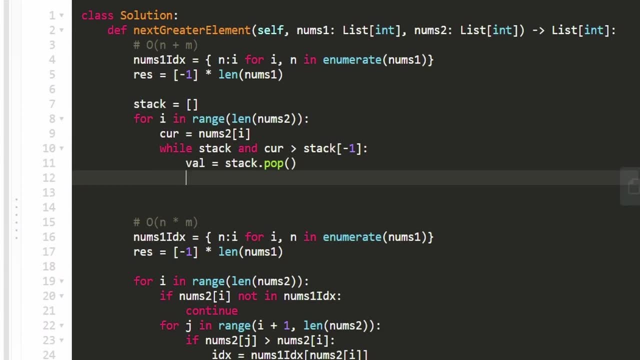 we want to pop from our stack and we're going to pop the value. we know that current is the next greater element of this value, So we want to find the index of this value. Thankfully, we have our index hash map to do that. So let's get the index of this value And then we can set that At that. 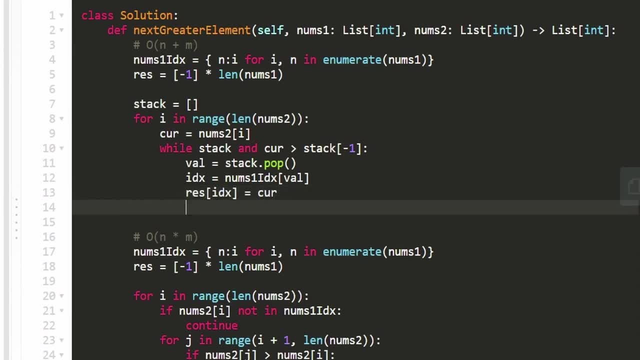 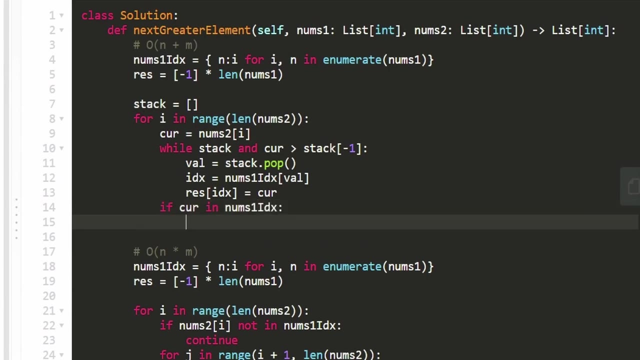 index, we can set the result, which is going to be Kerr, because Kerr is the next greater value. So pretty straightforward. After that is done, the question is: does Kerr show up in the first array? If Kerr is in nums one index hash map, that means it shows up in the first array. That means we: 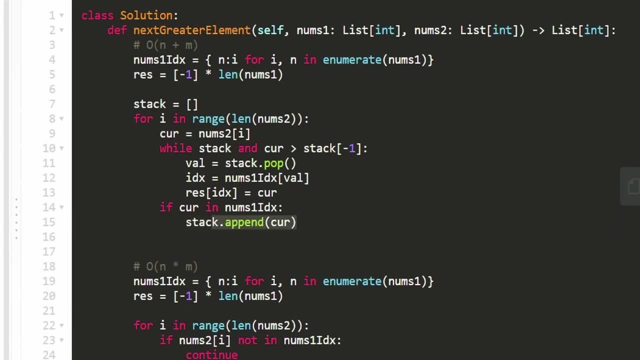 should add this to our stack Now. if it doesn't show up, then of course we just won't add it to the stack, because we don't need to. we don't need to find the next greater element of this stack or not of 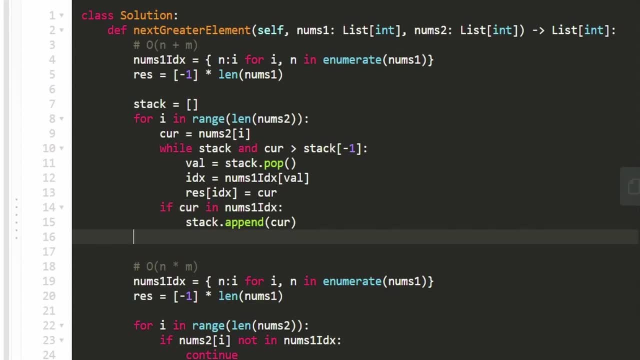 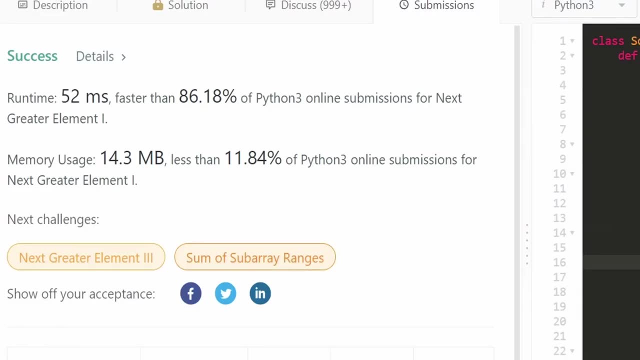 the stack of that value. But once that's done, that pretty much is the entire algorithm. we can go ahead and return the result And let's run the code to make sure that it works. And, as you can see on the left, yes, it does And it's very efficient. So I really hope that this was helpful, If it was.